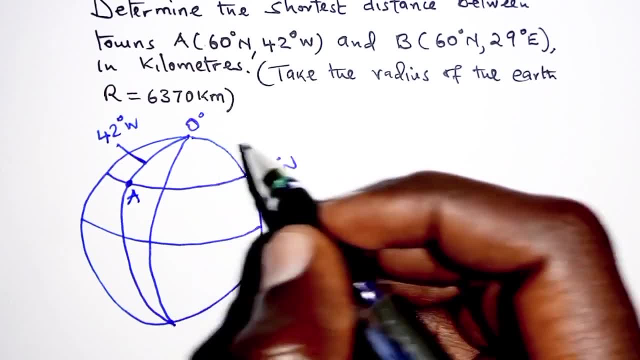 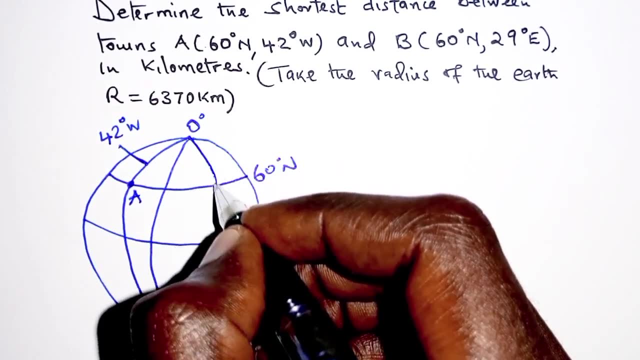 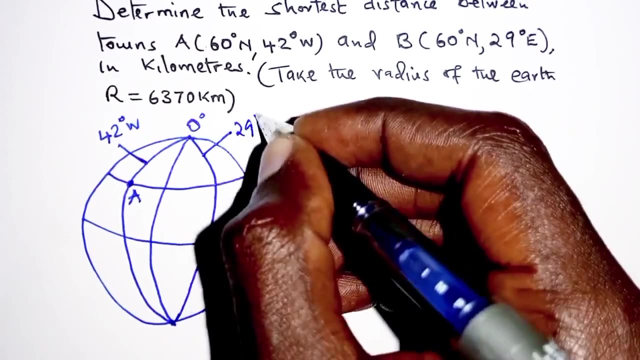 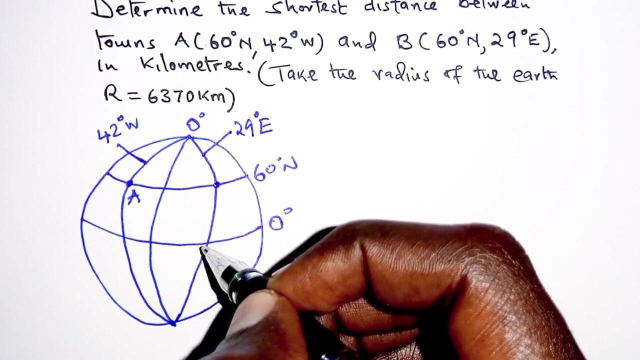 turn a. now for turn B. turn B lies on the same latitude, 60 degrees north, but 29 degrees east of the prime meridian. that is this longitude here, 29 degrees to the east of the prime meridian. so where the two meet, that is longitude: 29 degrees. 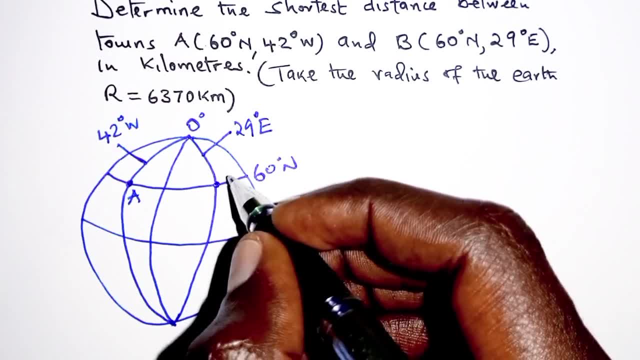 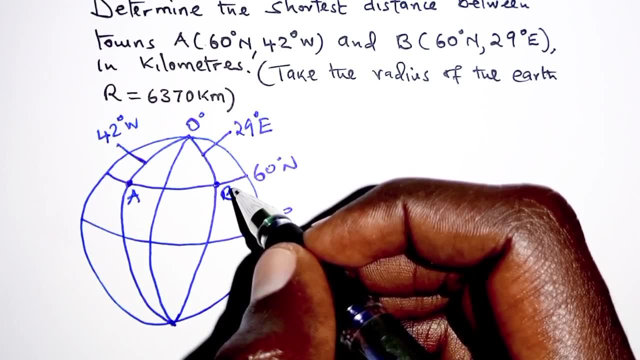 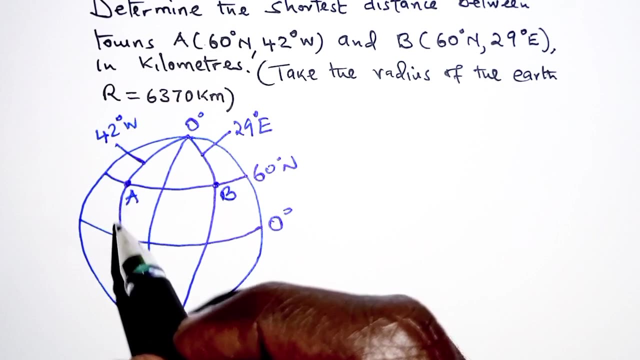 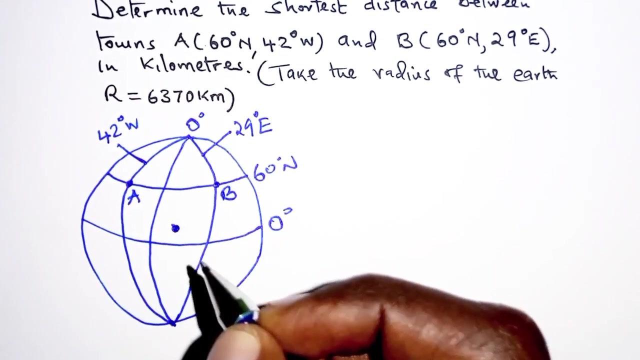 east and latitude 60 degrees north. that is the location of turn B. now, just as I had mentioned earlier on, the shortest distance between these two towns will be the distance along a great circle and we are going to consider a point, say here, to be the center of the earth, so that if we join, 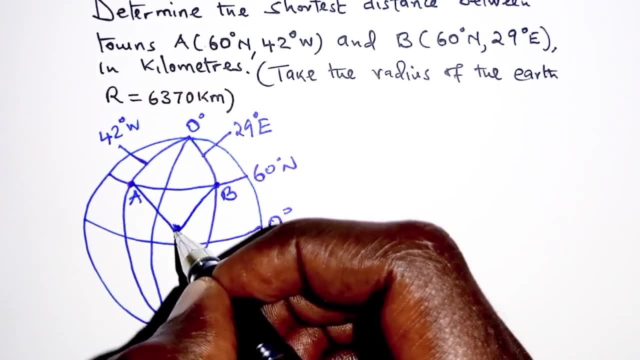 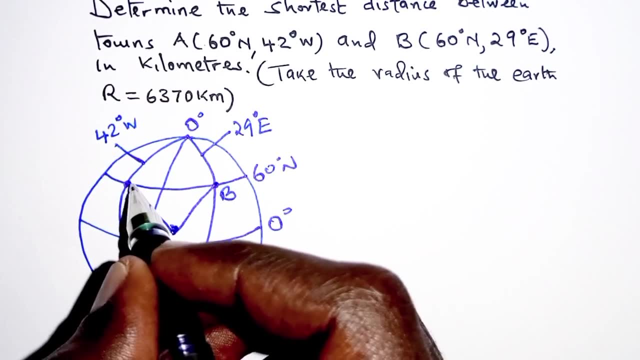 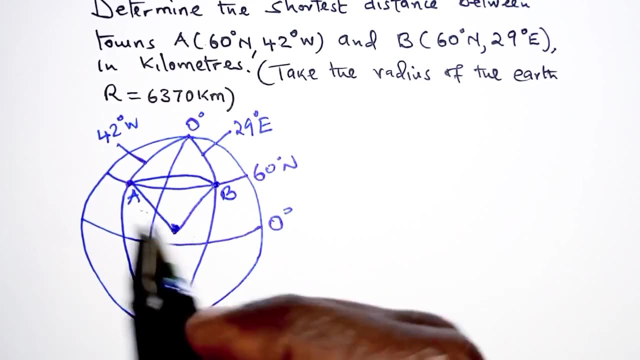 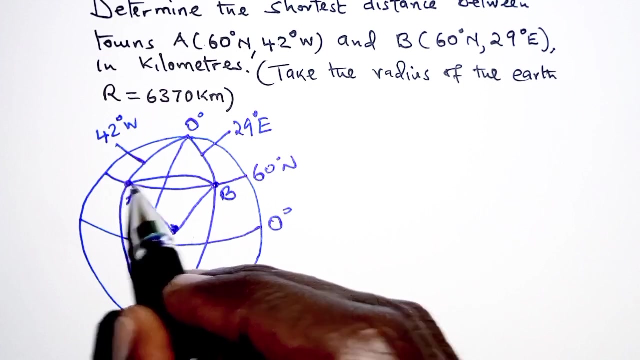 a to the center of the earth and B to the center of the earth. then we can come up with a sector by joining a to be, in this manner, form an act there. so we have this sector here now. this arc, joining a and B, which is part of this sector, is the shortest distance. now we make it the shortest. 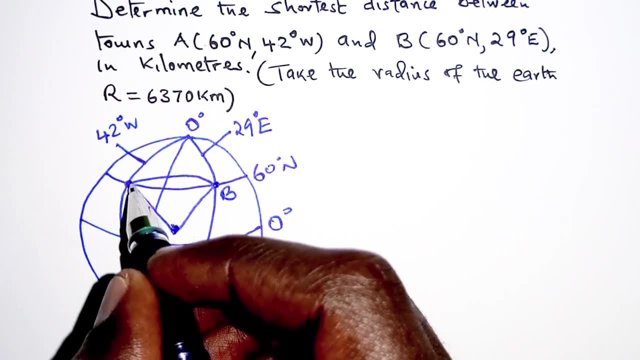 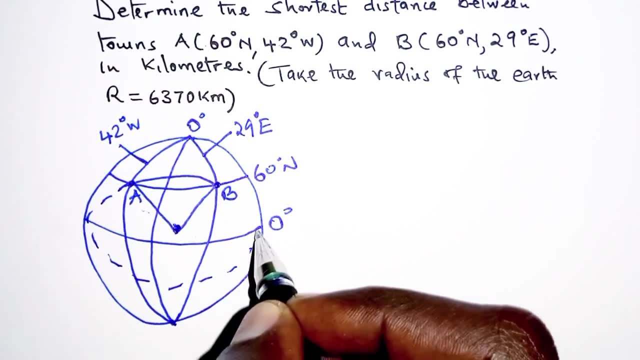 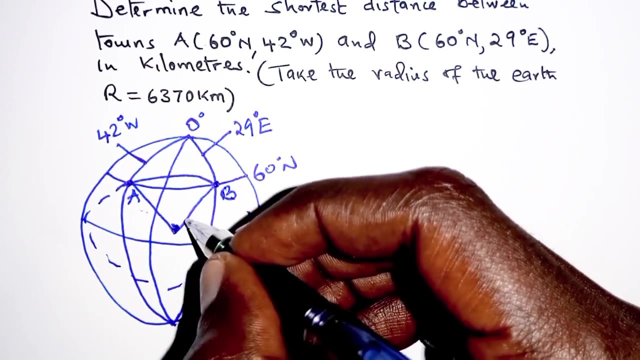 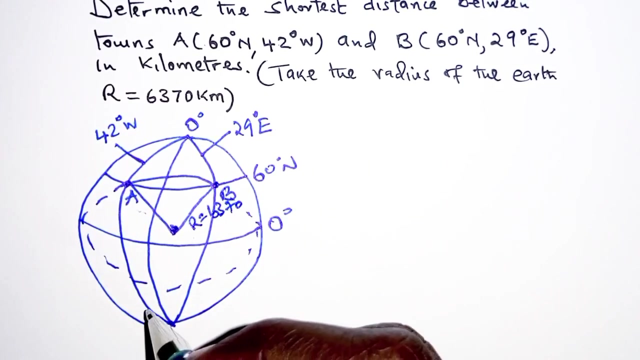 distance because it is part of a great circle. so we have this great circle. I'll have dotted now. I call it a great circle because its radius is the radius of the earth. so this radius here is 63, 70 kilometers. now in order to determine the shortest. 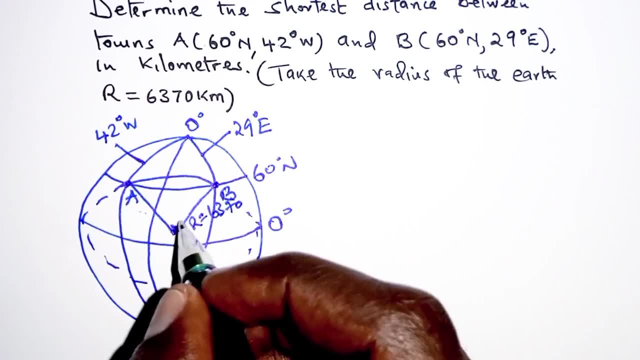 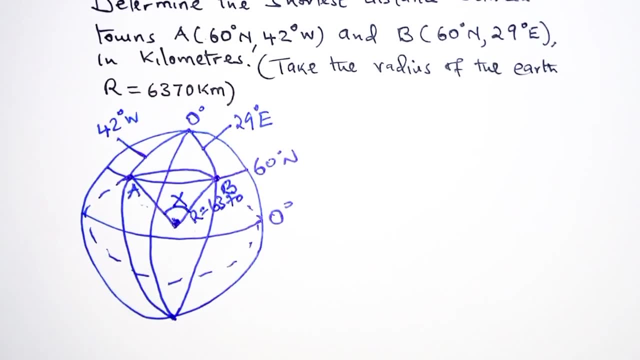 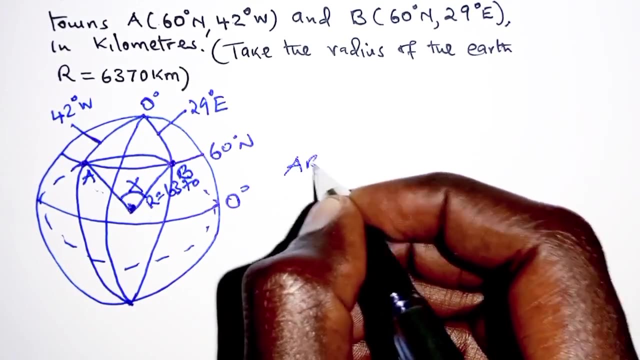 distance. that is the length of this arc a- B. we need to know the shortest distance. we need to know the angle it obtains at the center of the earth. let's call it X. well, before we get that X, we need to take note that the distance AB. 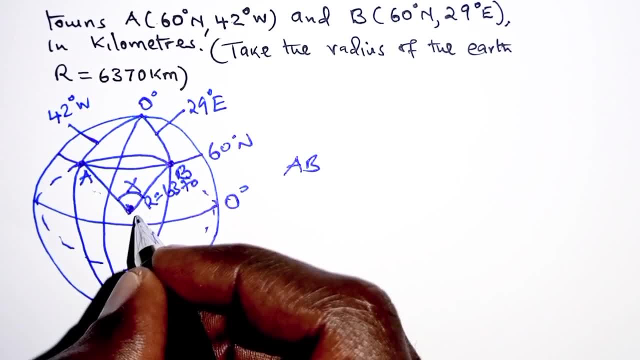 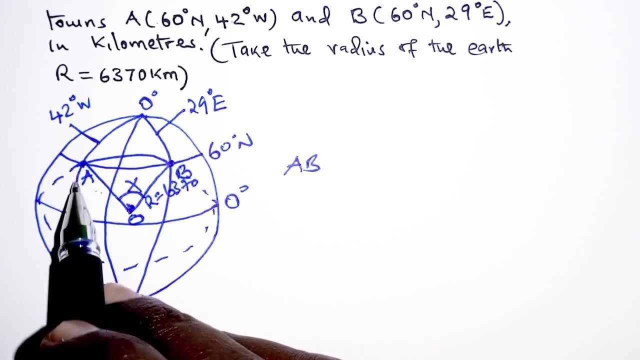 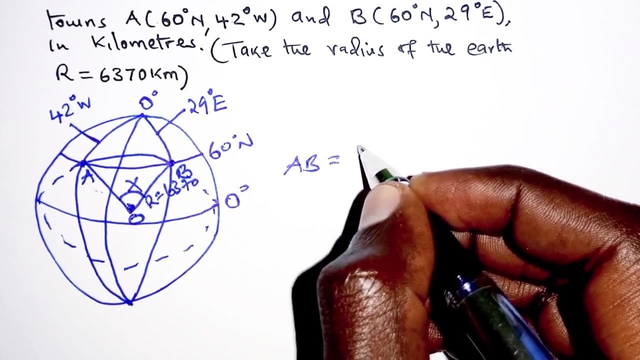 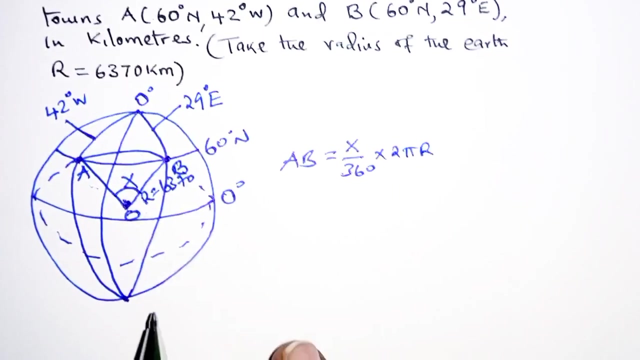 considering this sector. if we have the center of the earth as O, so consider the sector OAB. in order to get the length AB, that is, the earth length, then we'll use the formula X over 360 times 2 pi R, and therefore our task here is to determine the value of X, and X will be: 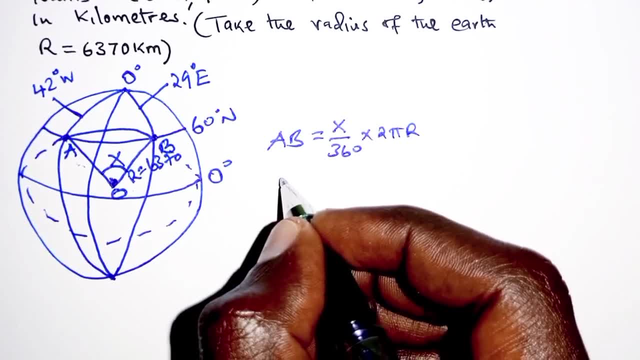 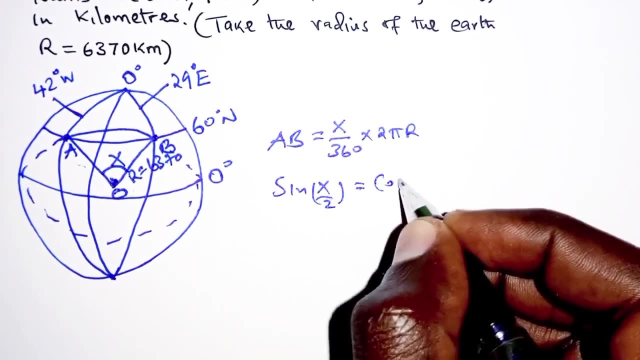 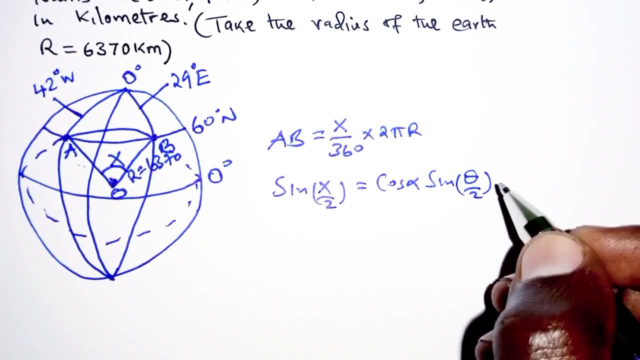 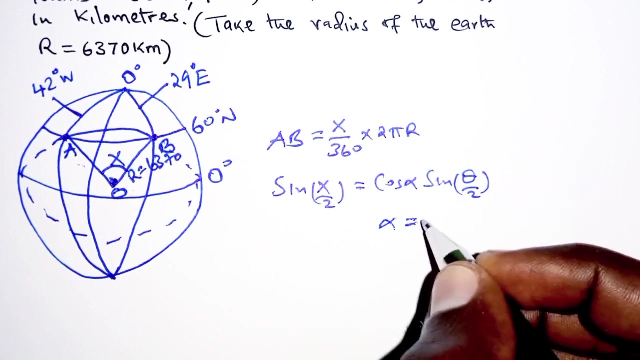 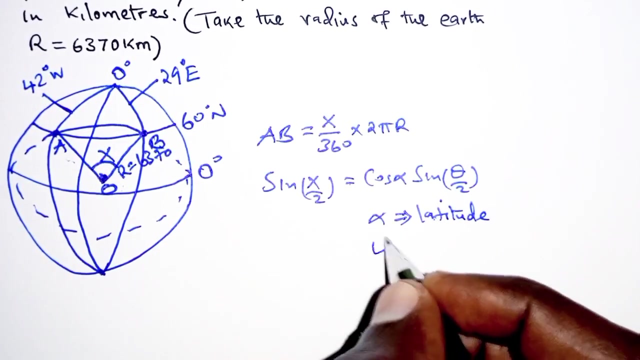 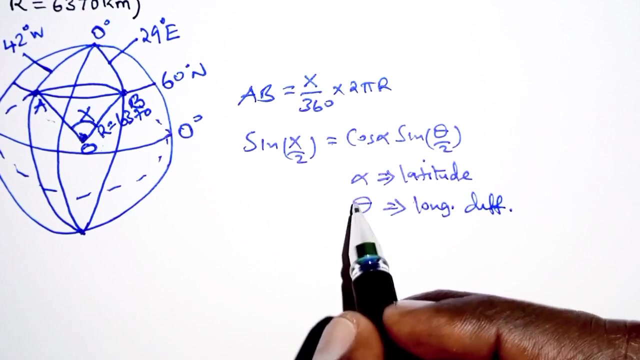 determined from this formula. so we say sine of X over 2 is equal to cosine of alpha, sine of theta over 2. so we'll take note that alpha here represents the latitude and theta represents longitudinal difference. so the first thing to determine is the value of the latitude and the. 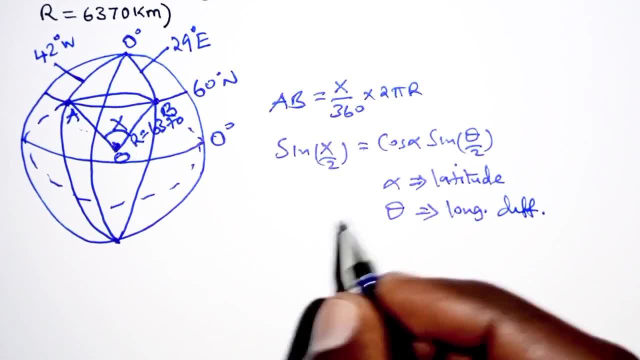 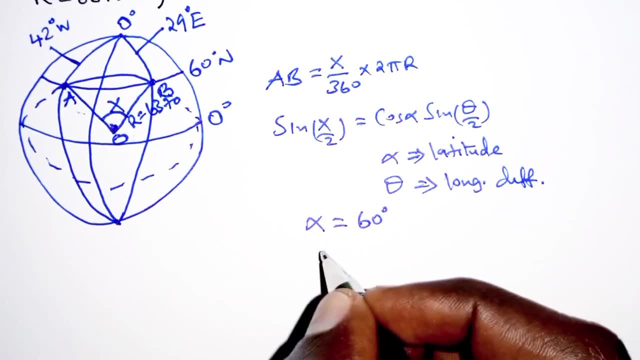 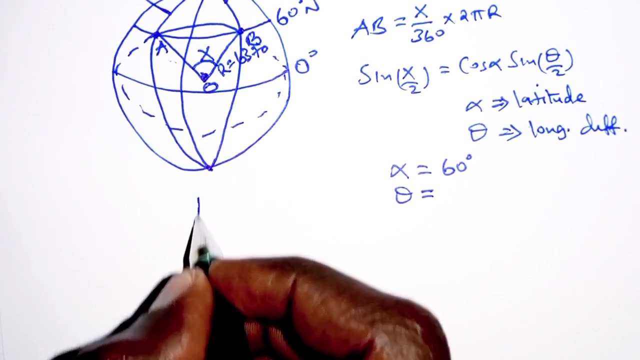 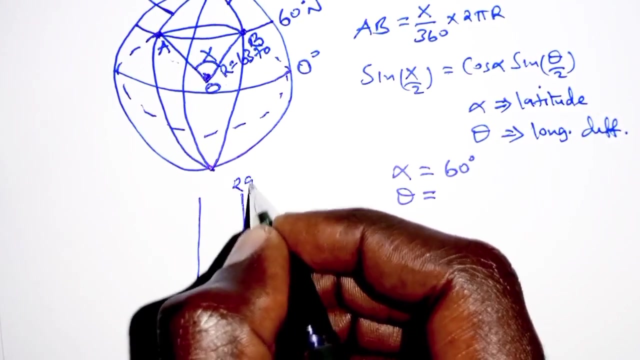 longitudinal difference. so the latitude from the question we've seen is 60 degrees north and the longitudinal difference will determine as follows: so we have the prime meridian and then to the east of the prime meridian we have this longitude, 29 degrees, that is east of the prime meridian. note that the prime 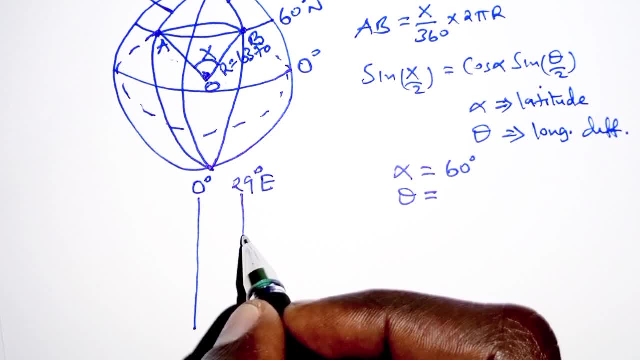 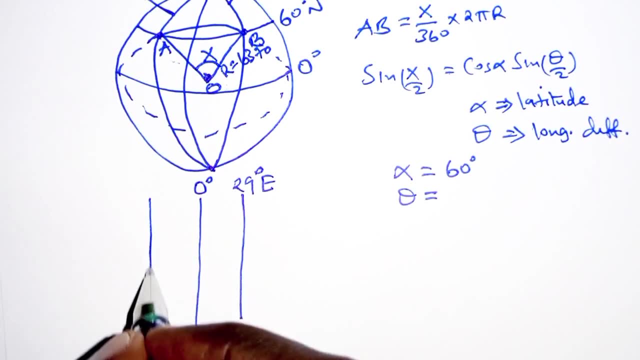 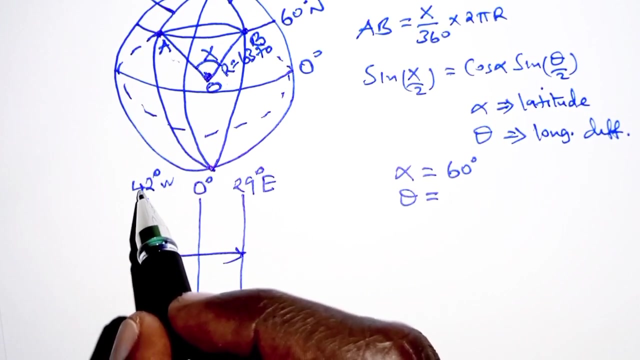 meridian is usually set at zero degrees. so to the east of the prime meridian we have longitude 29 degrees east, and then to the west we have longitude 42 degrees west. so the angle difference between longitude 42 degrees west and longitude 29 degrees east is the sum of 42 and 29. so that is. 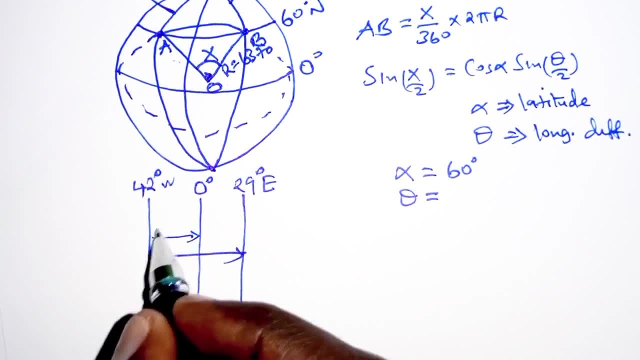 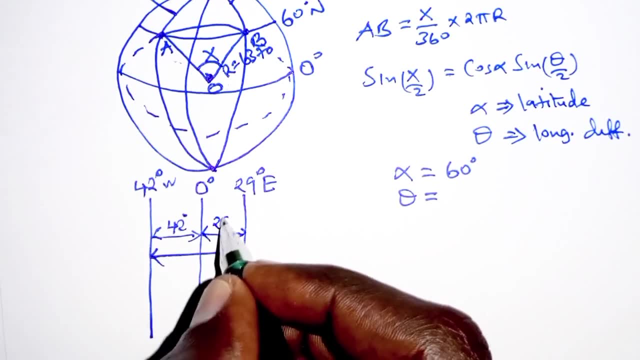 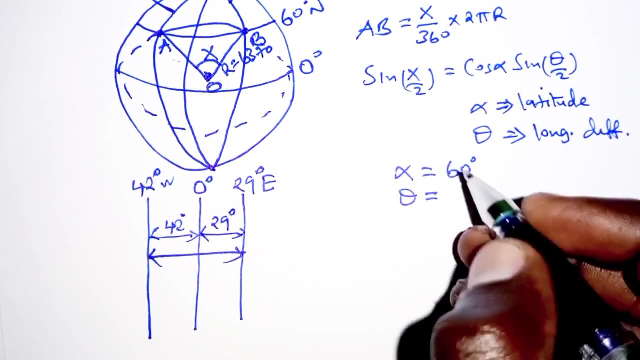 from 42 degrees west to the prime meridian. here we have 42 degrees. and from the prime meridian to longitude 29 degrees east, we have 29 degrees. so the total angle between the two longitudes is just the sum. so we're going to have 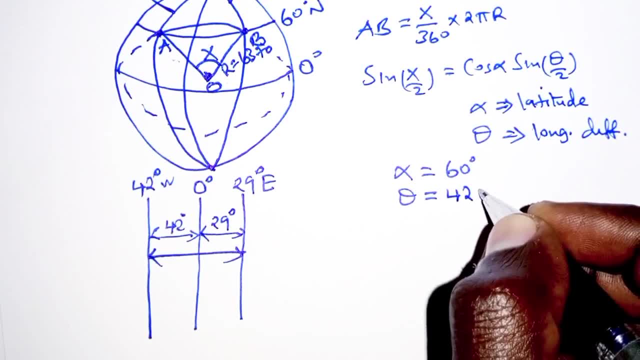 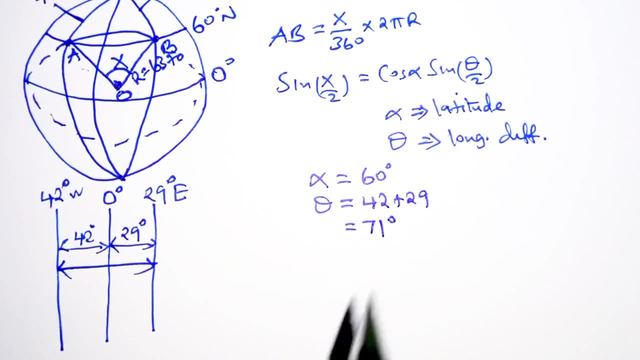 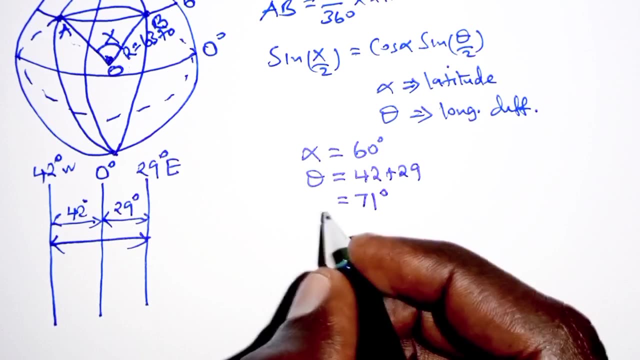 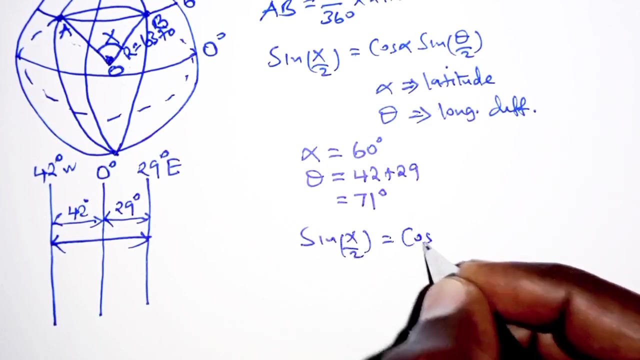 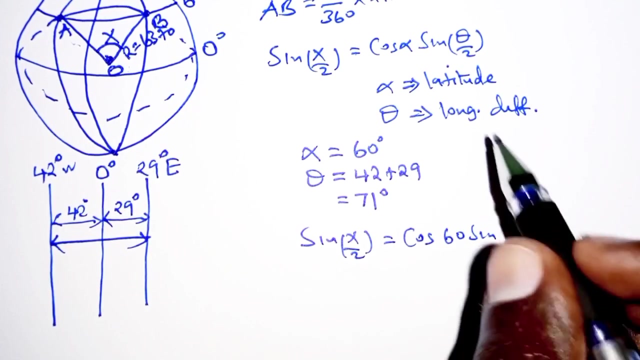 theta as 42 plus 29, so that is 71 degrees. with this you can now determine the value of X from this formula. so we'll do our substitutions. so we'll say sine of X over 2 is equal to cosine of alpha, and alpha is 60 times sine of theta over 2 and theta is 71 and therefore we divide. 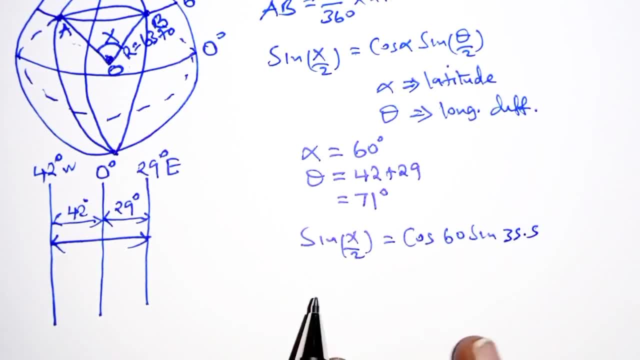 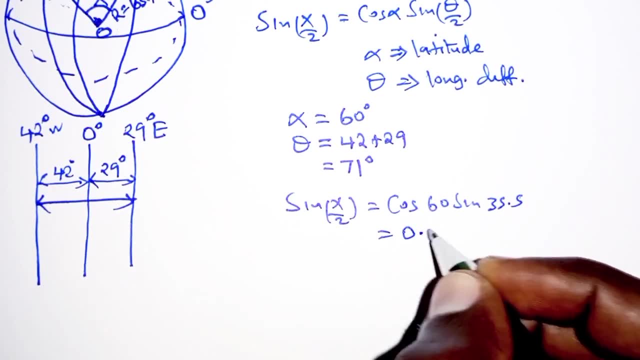 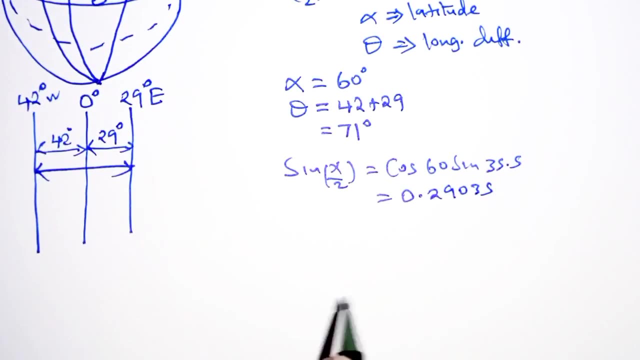 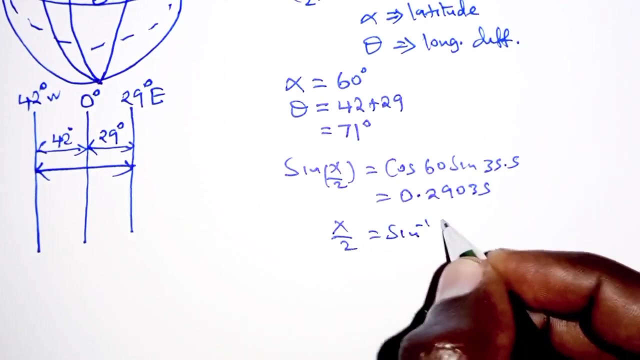 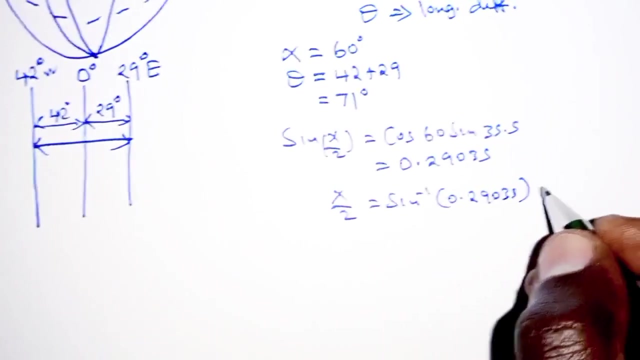 by 2, and that is 35.5. so from here, when we work out the right-hand side, we are going to get zero point 0.29035. from my calculator I'm able to get that, and therefore this means that X over 2 is the sine inverse of zero point 29035, and that is so we have 16.8. 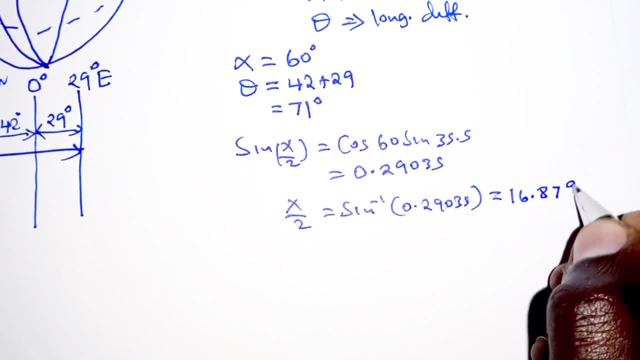 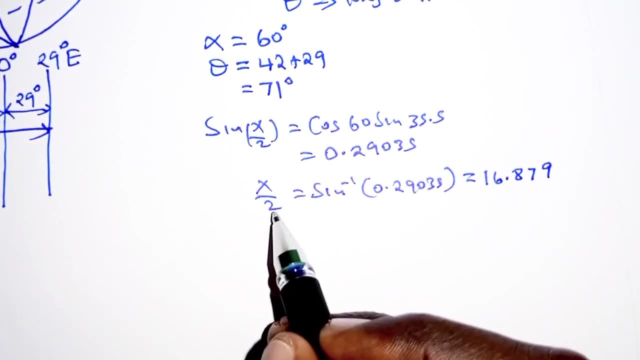 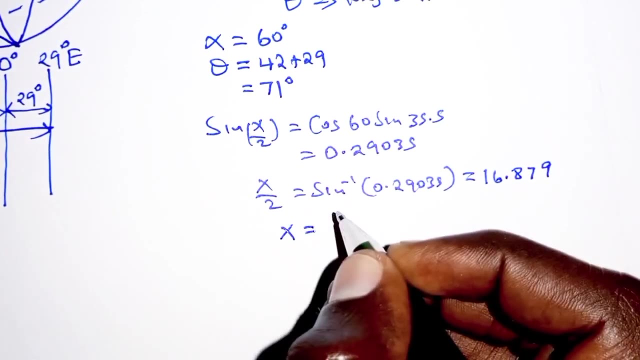 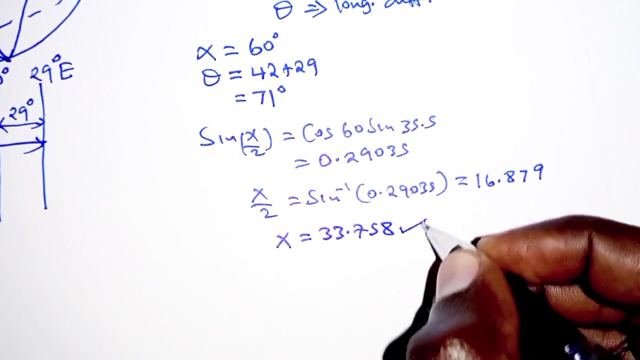 seven, nine. and then, Because we are looking for x, remember this is x over 2. Therefore, in order to get x, we multiply both sides by 2. Therefore, x is 33.758. So this is the angle subtended by this arc, arc AB. 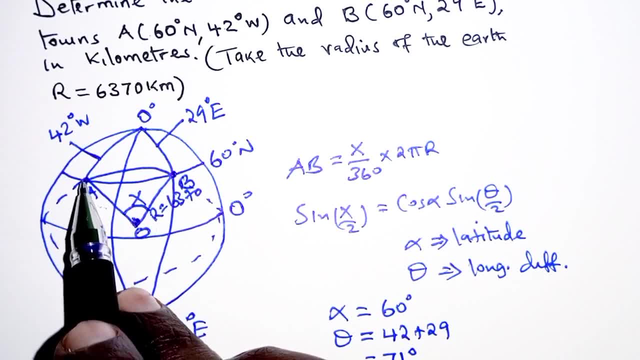 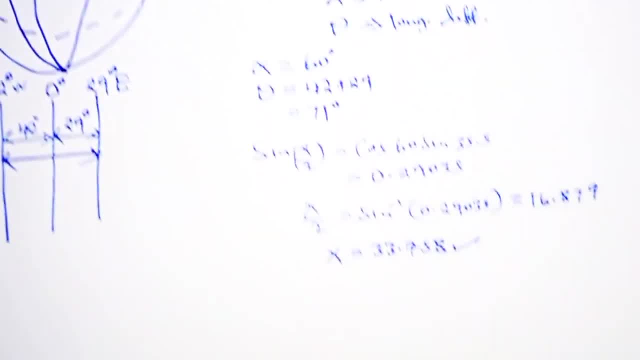 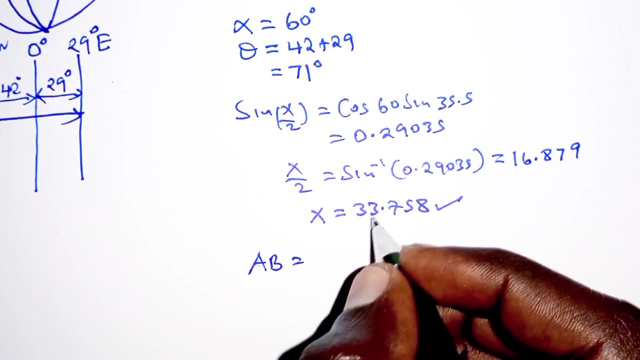 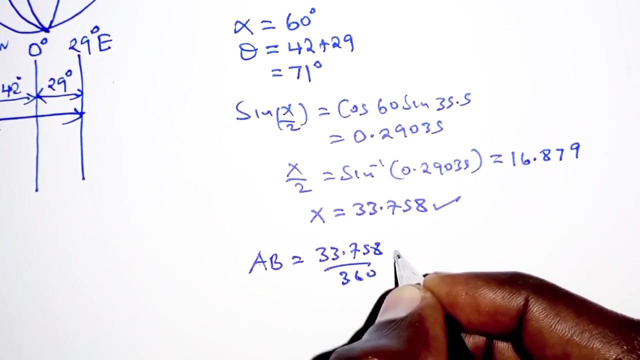 Which is the shortest distance between town A and B. So we are going to use it in this formula here. So let's write it: AB is equal to x over 360 And x is 33.758 all over 360 Times 2 times pi. 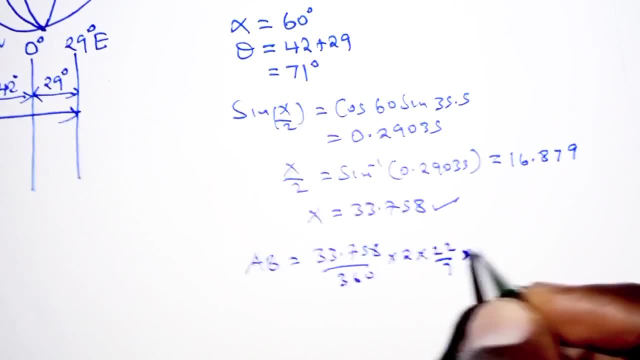 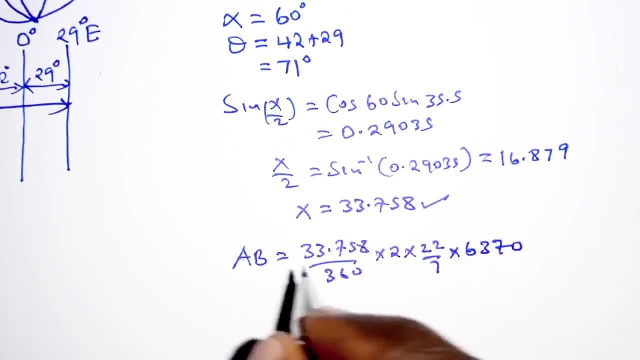 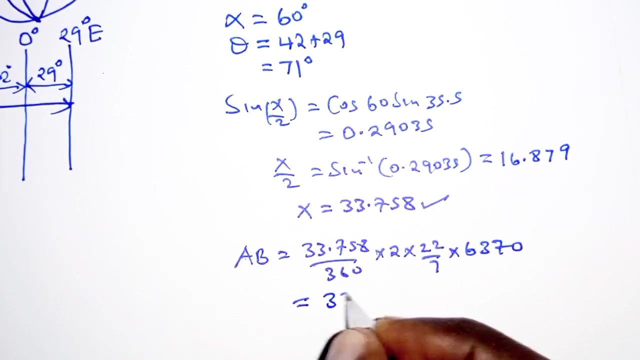 And pi is 22 over 7 Times r. r is the radius of the earth And that is 6,000, So we have 3370. So from my calculator, when I work out this, I am able to get 3754.64. 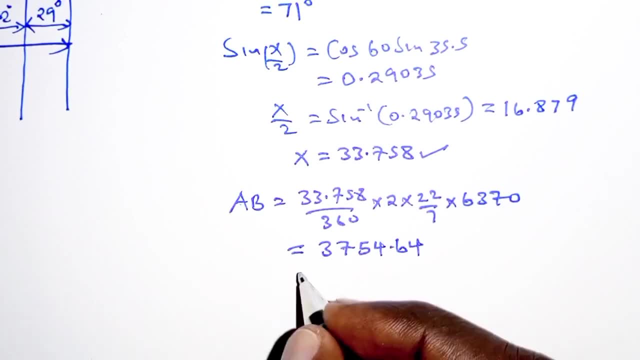 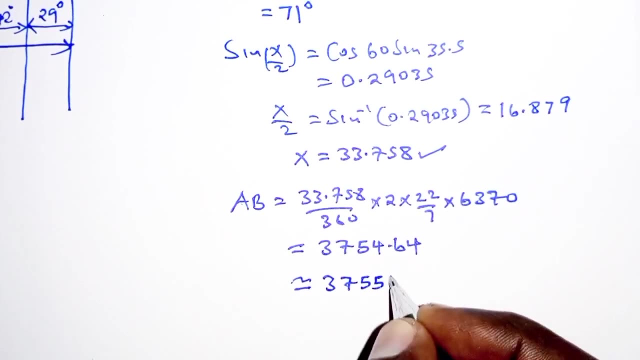 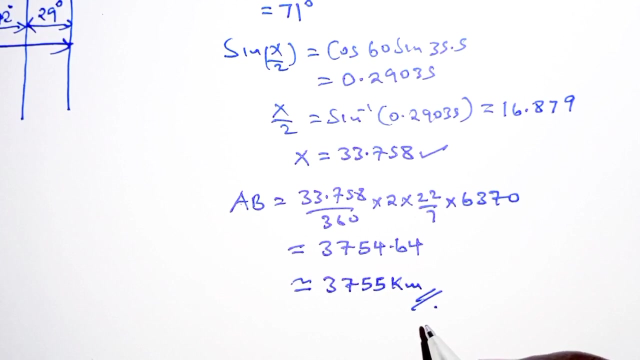 This is approximately 3755 kilometers And finally, we are going to use this formula here. Finally, we have the shortest distance between the two towns, Just as had been desired in the question. Thank you for watching. See you in the next one. 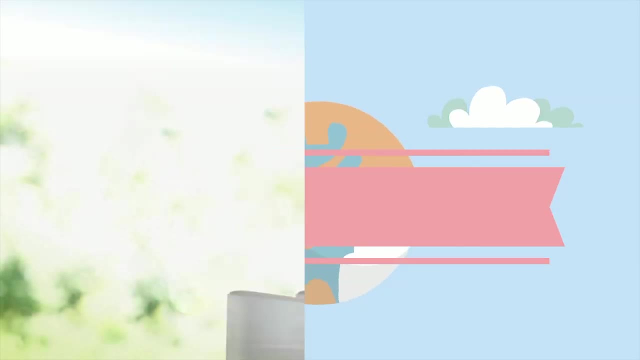 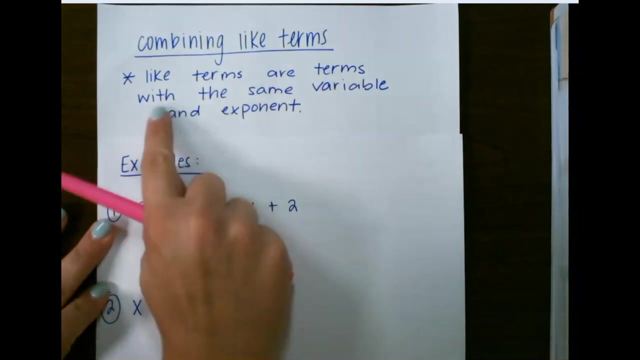 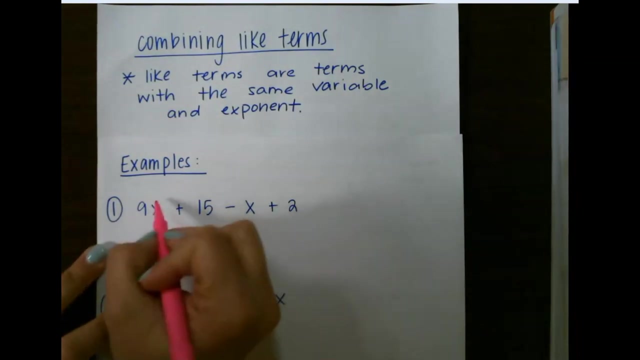 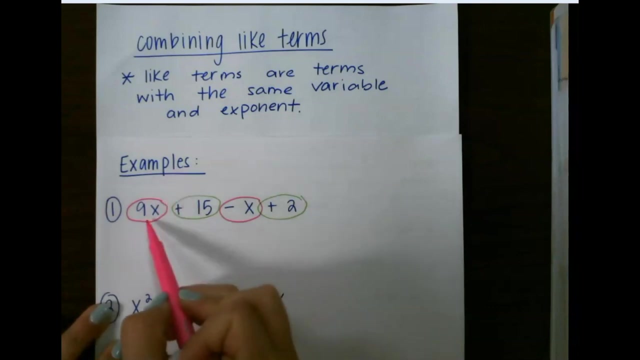 Combining like terms. Like terms are terms with the same variable and exponent. Let's look at our first example. I first want to label my like terms 9x and x and 15 and 2.. Notice that I circled the symbol in front of each term as well. So first 9x and x. 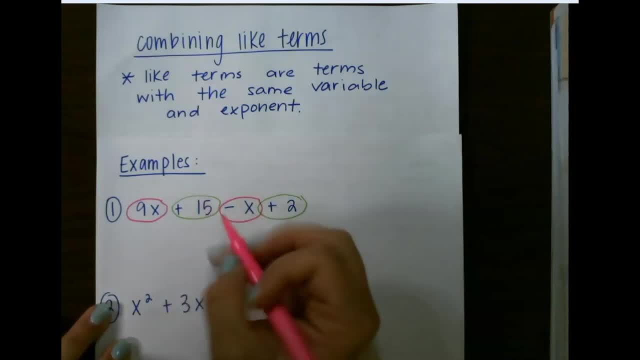 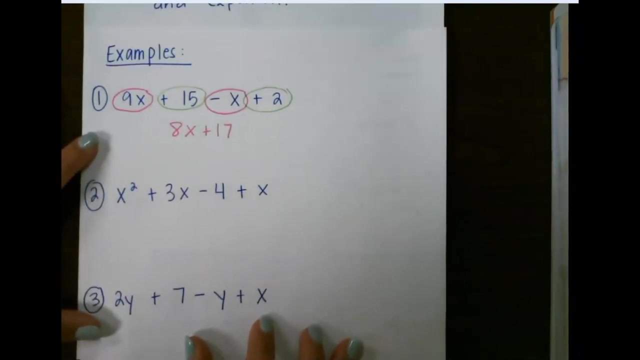 Since there is a subtraction symbol, 9x minus x will give me 8x. 15 plus 2, and this is positive- 15, is going to give me 17.. So that is our expression simplified. Looking at our next one: X squared. There are no other terms that. 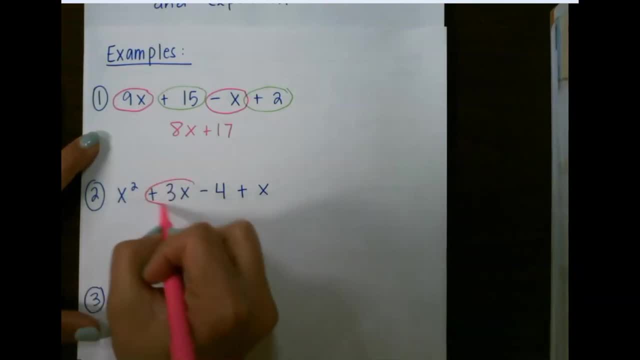 have x squared, So that cannot be combined with anything: 3x and x. We always want to start with putting our exponents first: 3x plus x would give me 4x, And then we just drop down minus 4.. 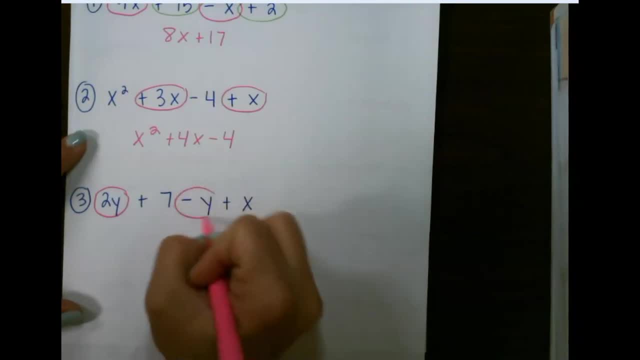 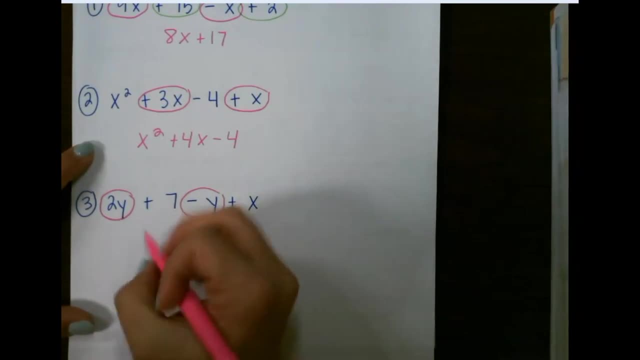 Lastly, we have 2y and y, and then 7 and x. There is nothing left to combine those with. So 2y minus y. We usually put them in alphabetical order, So I will put x first, And our plain regular numbers- these are called constants- will come last. Again, it is important to remember. 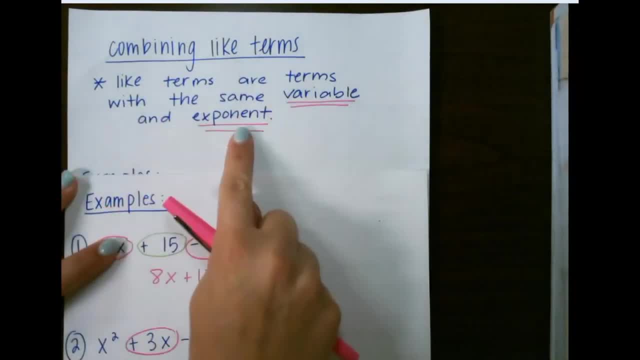 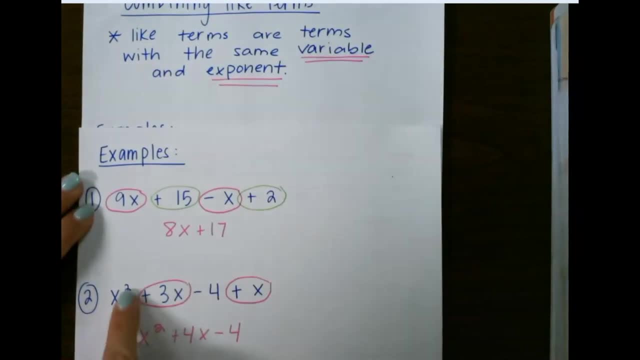 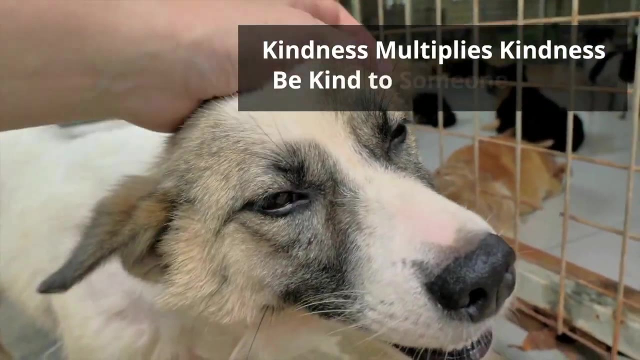 that like terms are terms with the same variable and exponent. Make sure you pay attention to the variable, which is the letter, and the exponent, which is the small number above it, like seen here. That is how we will put them in our